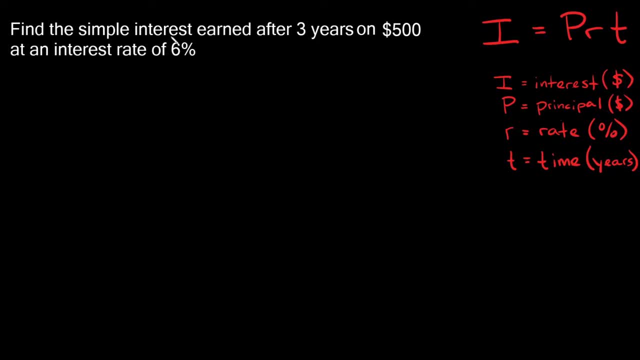 let's jump into this first example. So it says: find the simple interest earned after three years on five hundred dollars at an interest rate of six percent. Okay, so, as you can see, it's telling us to find the simple interest, right. So we don't know what the simple interest. 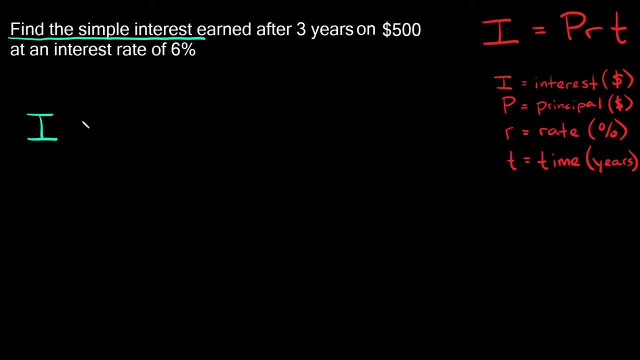 is. so we're looking for I in this case, right, and remember I is equal to PRT. So what are the values of PRT? Well, principal would be your dollar amount, right there? Okay, so it'd be five hundred, and then you're going to multiply that by R. What's R? It's the rate, right, and the rate in this problem is six. 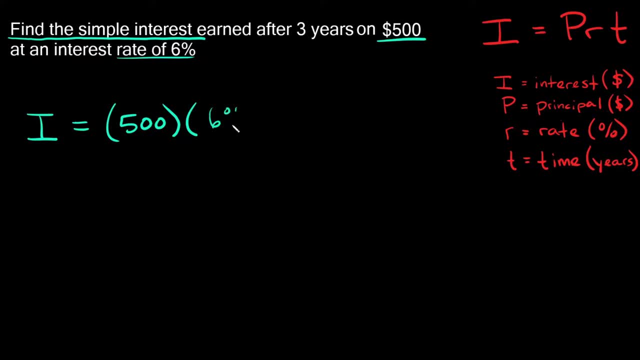 percent, Okay, but you don't put six percent here, Okay. you don't do that. You have to convert this percent to a decimal. So how do you do that? Well, an easy way of doing it is just dropping your percent sign. Okay, so we just have the number six. 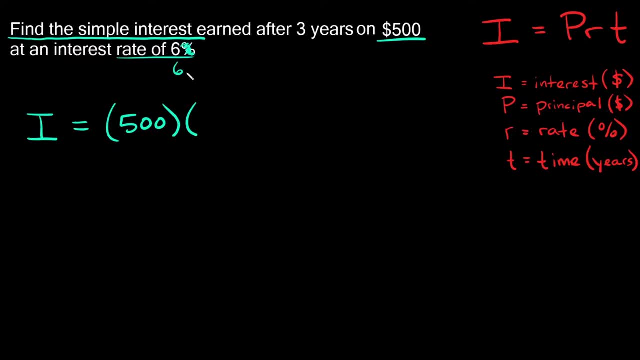 right. Where is the decimal on the number six? It's right there. Okay, so then just move it two times to the left: One, two. So that's where your decimal goes. Okay, and since we have a blank place value right there, you just put a zero. Okay, so six percent is the same thing as 0.06.. 0.06.. Okay so. 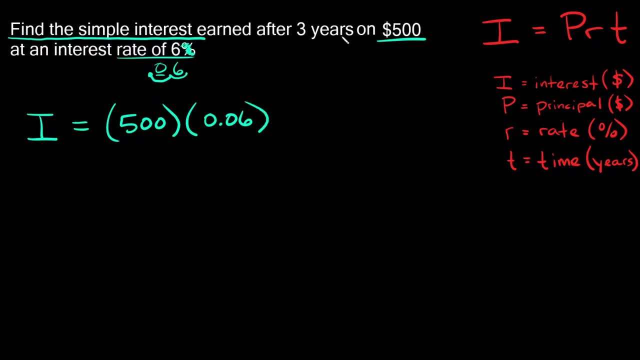 this is P, This is R, And then lastly T, Which in this case it's going to be three. right, because three years, Okay. so the simple interest is equal to 500 times 0.06 times three. So then you just plug that into. 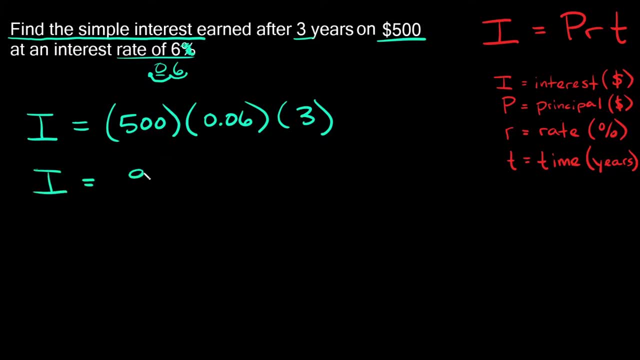 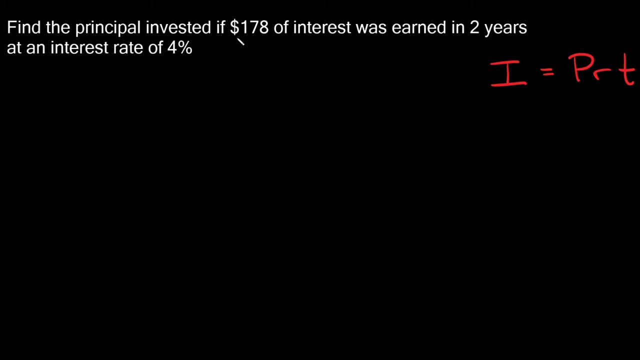 your calculator and then you would get that I is equal to 90.. Okay, 90, what? Well, what are the units? for simple interest? It's dollars, right? So your answer right here would be ninety dollars. Okay, so let's try a couple more. Now the problem says: find the principal invested if 178 dollars of 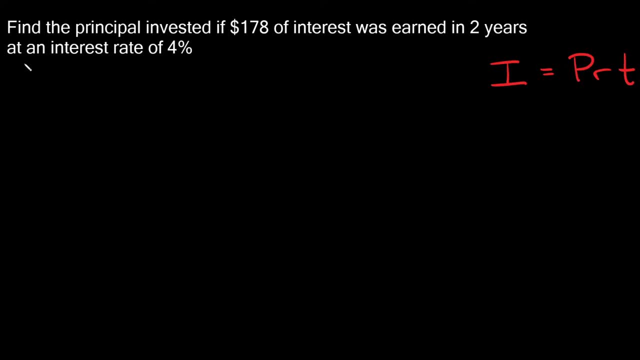 interest was earned in two years at an interest rate of four percent. Okay, now, sometimes these problems can get a little confusing, So if it helps you, you can write out right off the bat what each one is equal to, Okay, and then you can plug it into the formula after. So here it says. 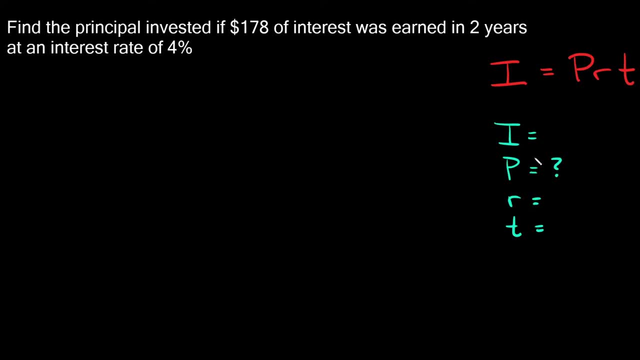 the principal, right? So we don't know what the principal is. So what do we know? Well, it says $178 of interest. okay, So that means I would be 178,. okay, Was earned in two years, right? So that means time is equal to two years. 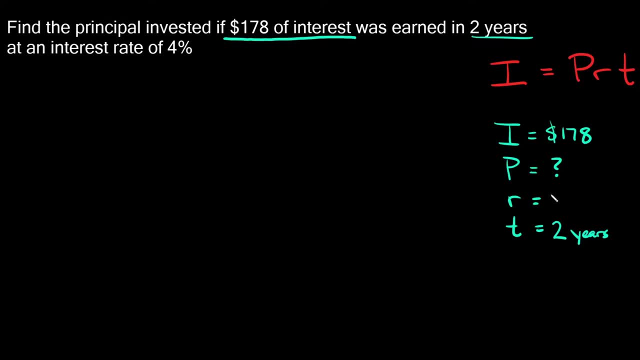 At an interest rate of 4%. so your rate right here would be 4%. Okay, but remember, when we plug it into the equation it has to be a decimal. So, following the same little trick I taught you in the last problem, as a decimal this would be. 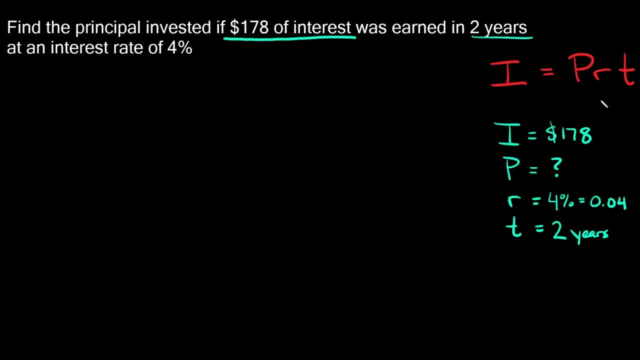 0.04.. Okay, so now let's plug these numbers into our equation, right there. So I equals PRT, So I is 178, and that's equal to P, which we don't know right now, right Times R, which is .04 or 0.04,. 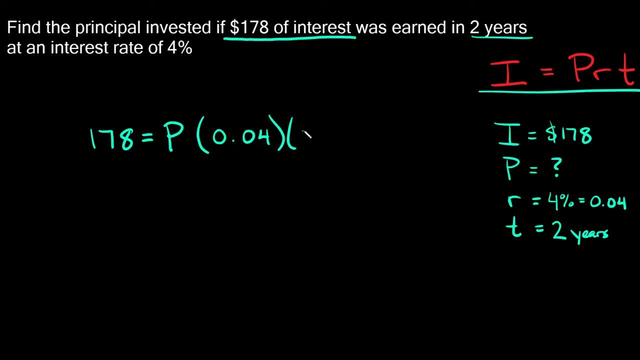 times the time, which is two years, So two. Now how do I solve for p right here? Well, one thing I'm going to do first is simplify my numbers a little bit. So I'm going to say: 178 is equal to p times this. 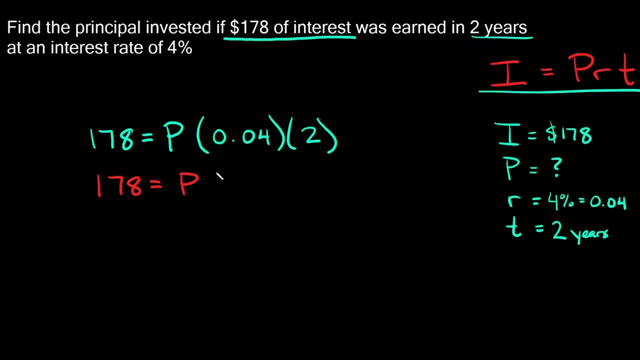 right. So what is 0.04 times 2?? Well, that would be equal to 0.08.. Okay, so, now that I simplified this a little bit, I have to solve for p, right? So that means I need to get rid of this 0.08.. 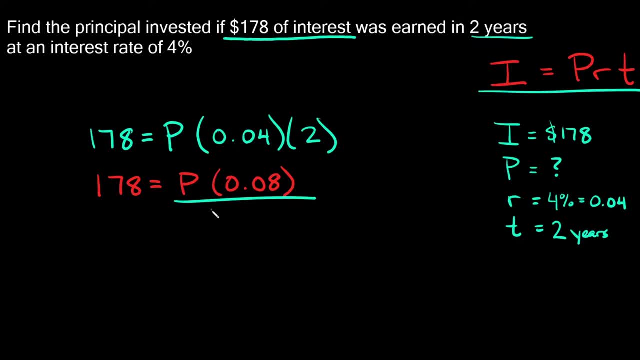 So since we're multiplying here, I'm going to divide by 0.08.. Okay, and what you do to one side of the equation, you do to the other, right. So divide on this side by 0.08 also Okay. so these cancel each other out. so then I'm just going to be left with p on this side of the equation. 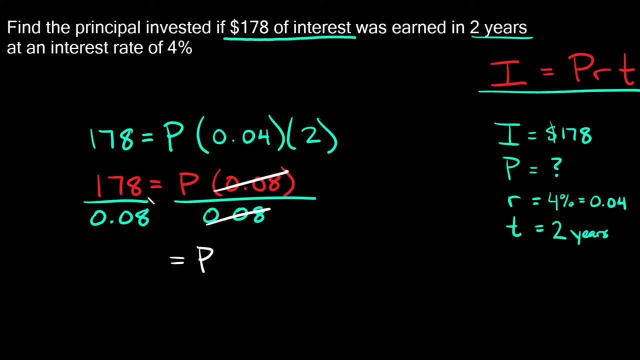 and then that's equal to 178 divided by 0.08.. So I'm going to divide by 0.08.. So I'm going to divide it by 0.08, which if you plug that into your calculator, you would get 2,225.. And what are? 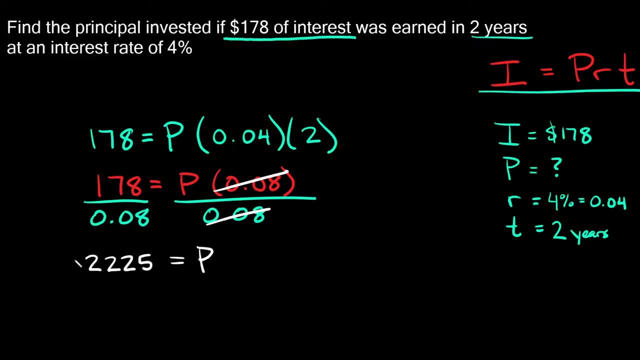 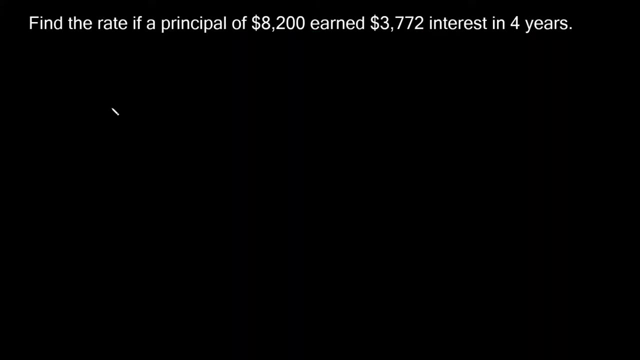 your units for the principle. Well, remember, it's dollars, right? So the principle right: p is equal to 2,225 dollars. So that would be your answer, right there. Okay, so let's do one more. Okay, so this last problem says: 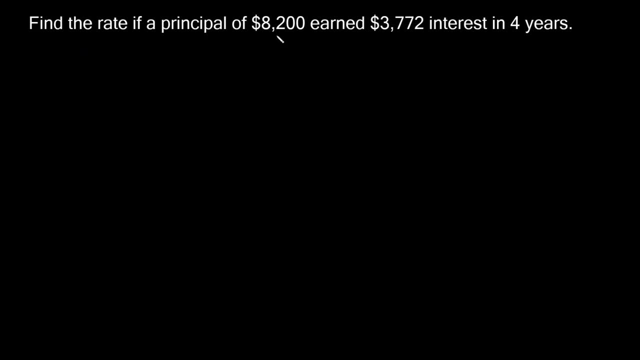 Okay. so there's obviously a lot of information right off the bat, but just always start at the same spot. Okay, just remember. this is your equation, right? I is equal to p? r t. Okay, so now let's just fill in things that we know. So here it says: find the rate. Okay, so that means. 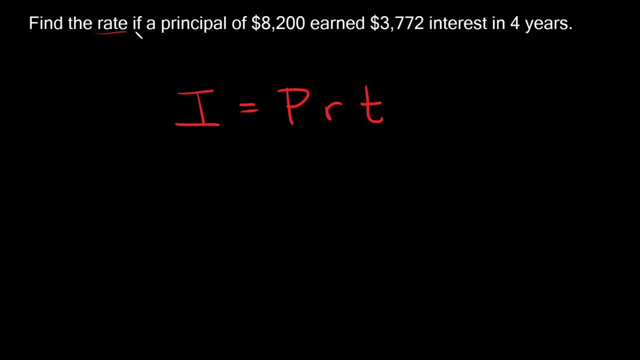 we don't know what the rate is right. That's what we're going to be looking for. And then it says: if a principal of 8,200 dollars, Okay, so my principal is going to be 8,200.. Okay, and. 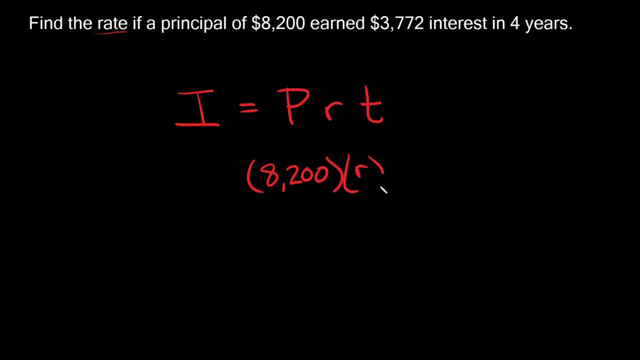 we're multiplying that by r Right, which is unknown, so I'll leave it as r. And then what else does it say here? earned $3,772 dollars interest. Okay, so i is equal to 3772.. Okay, so i is equal to. 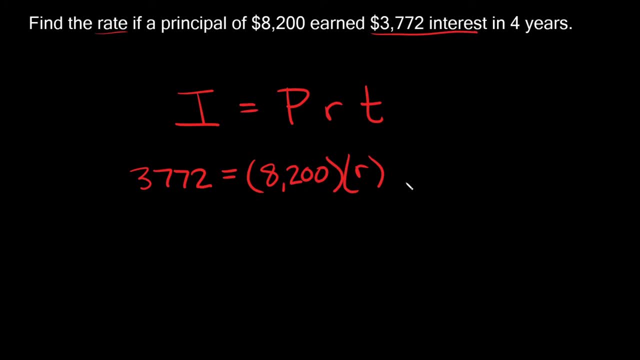 Okay, so I is equal to PRT. And what is T? Four right, Four years, All right. so let's simplify some things. So I'm going to say 3,772 is equal to Now what's 8,200 times four. 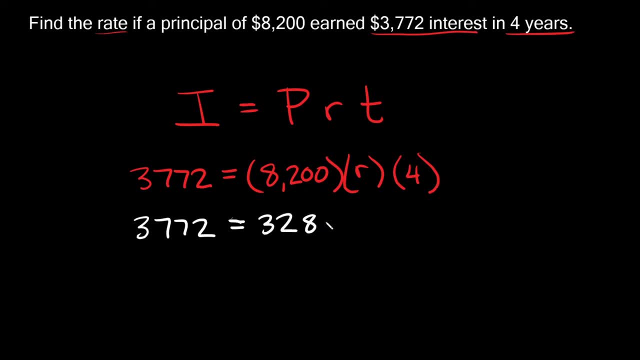 That would be 32,800.. Okay, and remember, we're still multiplying by R, right here. right, We're still multiplying by R. Now, how do I solve for R right here? Well, I'm going to have to divide by whatever I'm trying to get rid of. 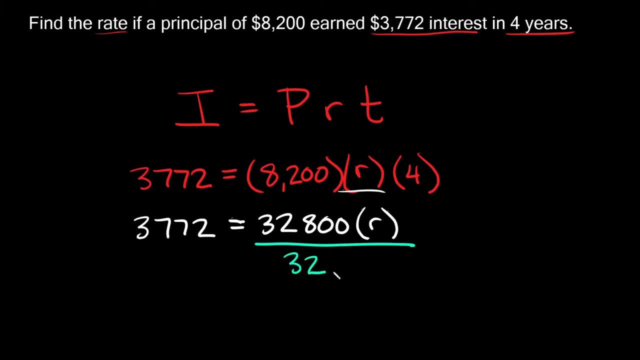 which would be the 32,800,, right, 32,800.. And what you do to one side of an equation? you do to the other: 32,000 divided by 32,800.. Okay, so now these cancel out. 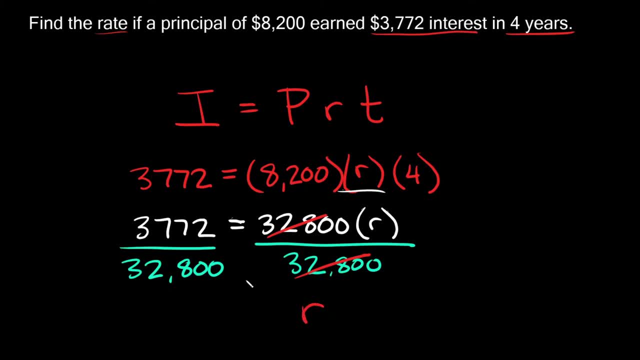 So we're just going to be left with R on this side of the equal sign, And then that's equal to 3,772 divided by 32,800.. So what is this equal to right here? Well, if you plug that into your calculator, you're going to get 0.115.